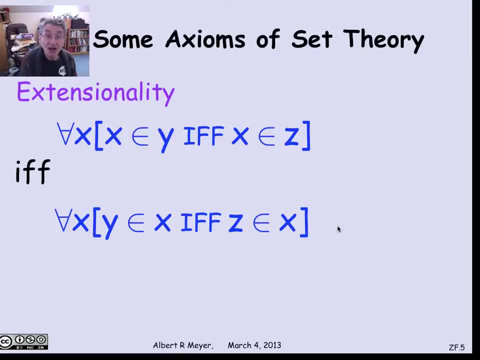 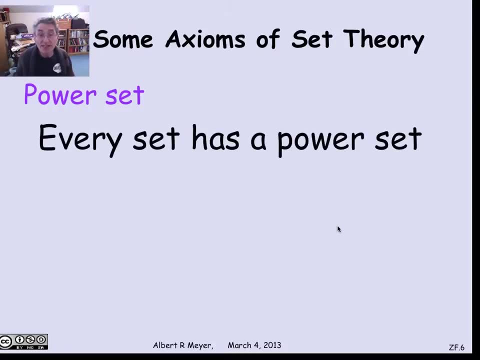 So that is one of the basic axioms of set theory, maybe the starting one. Another one is the power set axiom, which simply says that every set has a power. How would you say that in the language of predicate set theory? Well, you'd say that for every x, there is a p, which is going to be the power set of x. 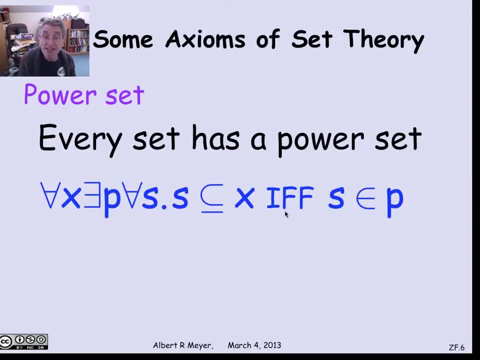 such that for every set s, s is a subset of x if, and only if, s is a member of p. Remember, we know how to express s as a subset of x in the language of predicate calculus mentioning only membership. So this is a good axiom that says, yes, there is a set p consisting of precisely the subsets of x. 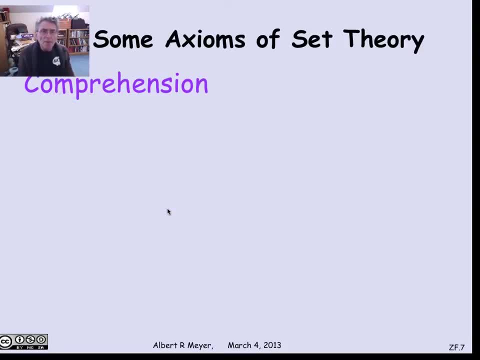 and that set p is called the power set of x. When you're trying to deal with the Russell's paradox kind of issue, where you define a set of elements or a collection of sets that satisfy some property, the safe, conservative version of saying that a set of elements that satisfies some property really is a set, 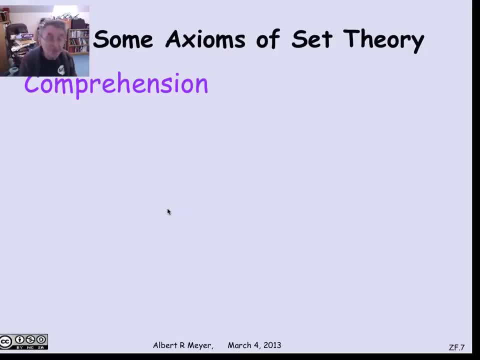 a collection of elements that satisfies some property really is a set. the comprehension axiom is a simplification. It's a simple version of an axiom that allows you to do that. So basically, it says that if s is a set and p of x is an arbitrary predicate of set theory. 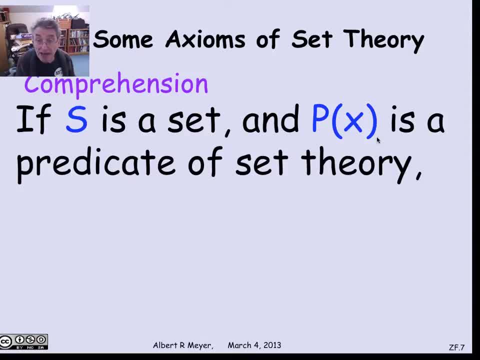 which might in fact be one of these dangerous things like x is not a member of x. nevertheless, if you look at those elements in the set s that satisfy p of x, that's a set. In other words, the set of x in s such that p of x is a set. 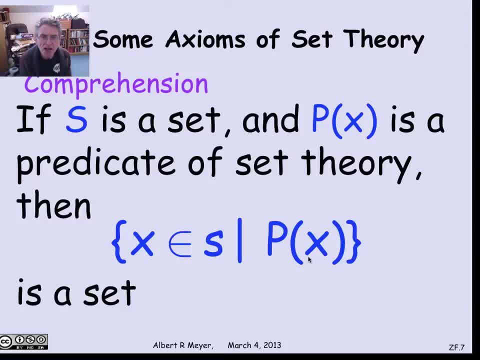 it means that any definable collection of elements within a set also form a proper subset. And the reason why this matters is, remember, if I just talked about, not the set of x in a particular set, s that satisfy p of x. if I just talked about the collection of x's that satisfy p of x. 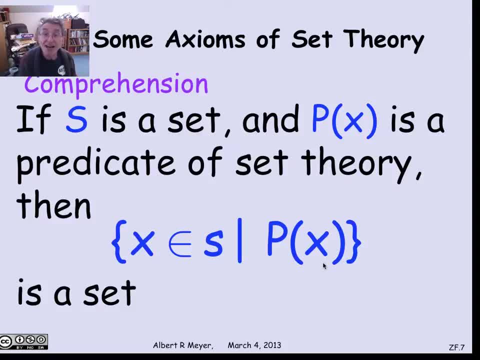 that's when I start getting into Russell's paradox areas. when I declare that the set of x, such that p of x, is a set, it's a set for unrestricted p of x. But all I need to do is put a bound on the elements that x ranges over. 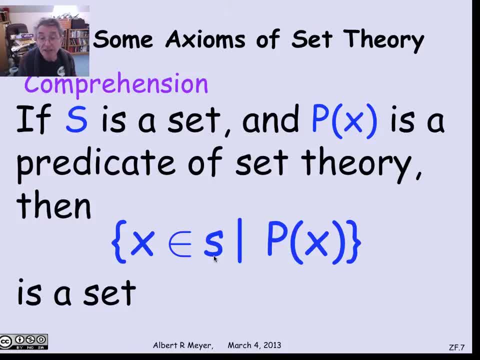 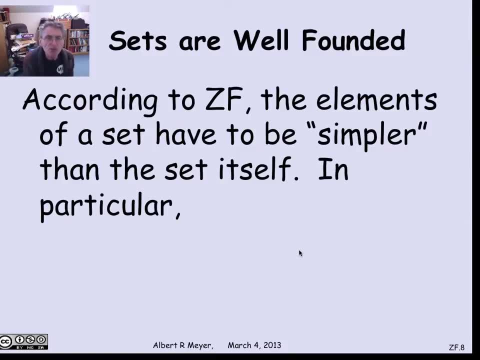 that x is a member of some particular set, then it's safe to take all of those x's that satisfy p of x. Now, another particularly interesting axiom of ZF, which addresses this issue of self-membership and self-reference, is that the intuitive idea that the elements of a set have to come before the set itself, 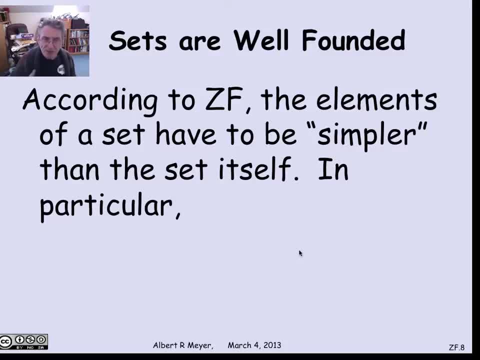 they have to be simpler- simpler than the set itself, If you think about sort of building up a set from successively simpler elements to more complicated ones. in particular, you can't have a set be a member of itself, because then it's not being built from things that are simpler than it is. 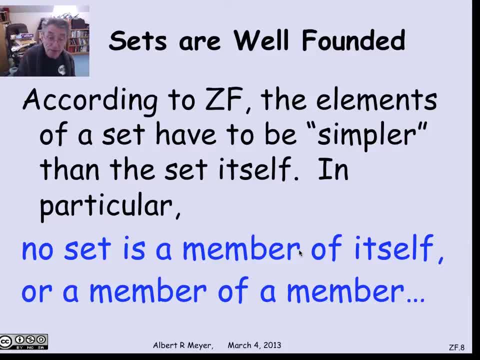 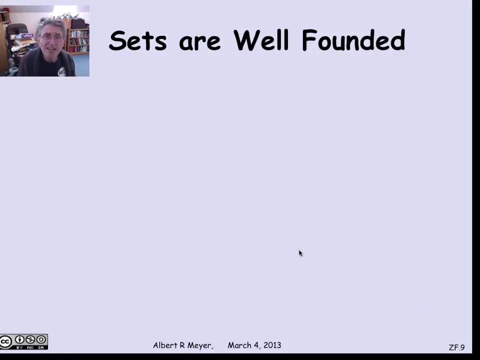 or that came before it is. In fact, you can't even have a set that's a member of a member of itself. All of that kind of indirect membership is forbidden. Now, how do you say that as a nice axiom? Well, there's a very elegant way to do it. 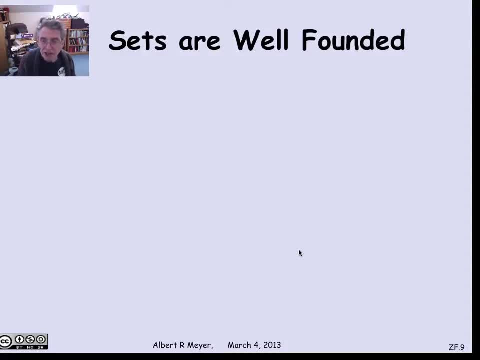 and that is to say that all sets are well-founded under membership, which means that you can't find an infinite sequence of sets where each one has the next one. as a member, Let's give a precise way to formulate that. It's also good practice with the formulas of set theory. 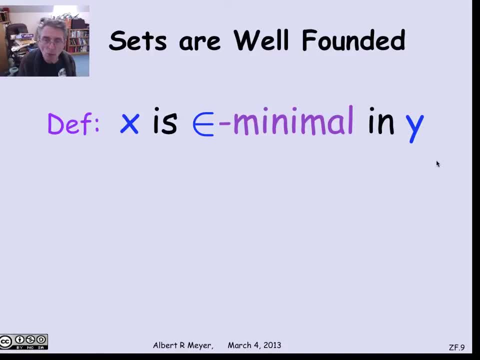 Let me say that x is membership minimal. epsilon minimal in y means that x is a member of y, but there's no element of y that's a member of y. There's no element of x that's also in y. In other words, x is built out of things that are not in y. 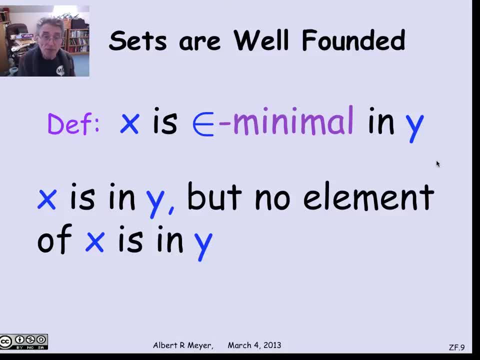 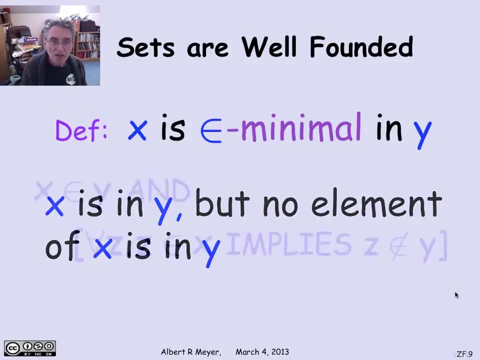 but x itself is in y. So x kind of comes before any of the other elements in y. It's built out of non-y stuff. So, to say this with a formula, we could just say that x is in y and for every z, if it's in x, then it's not in y. 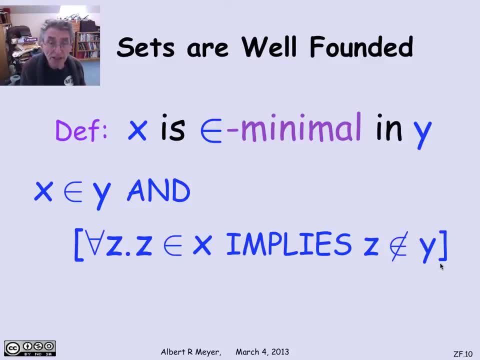 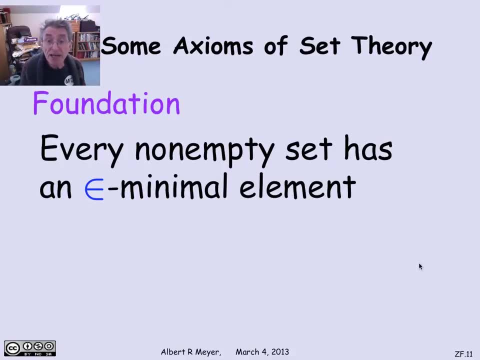 So that's the definition, that x is membership minimal in y. And then the basic axiom of ZF, called the foundation axiom, simply says that every non-empty set has a membership minimal element. This is actually a kind of generalization of the well-ordering principle that 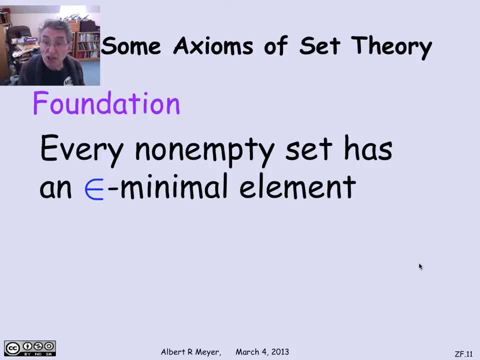 says that every non-empty set of non-negative integers has a least element. This is a direct analogy. Just as the well-ordering principle for integers implies that you can't have an infinite decreasing set, a decreasing sequence of non-negative integers, the foundation axiom actually implies 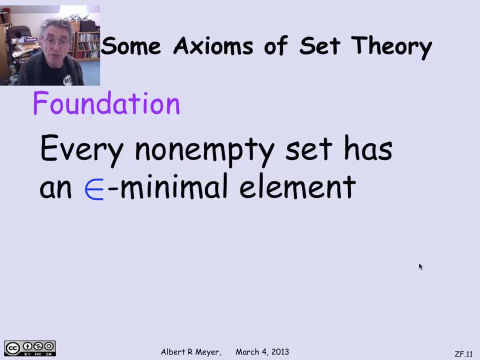 that you can't have an infinite sequence of sets, each of which is a member of the previous one. And here is a formula that's asserting foundation for every x. If x is not empty, that implies that there is a y, such that y is membership minimal in x. 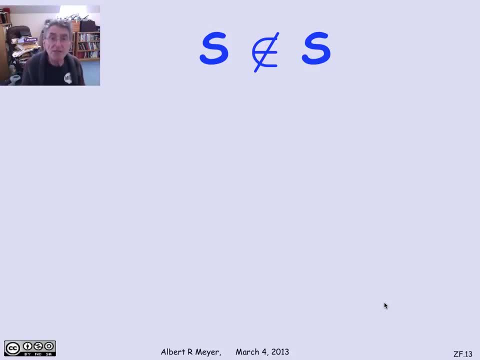 Well, what has the foundation got to do with membership? Well, the foundation Axiom will very quickly let us conclude that no set is a member of itself. How does that work? Well, suppose that you are interested in some set and you'd like to verify that this set can't. 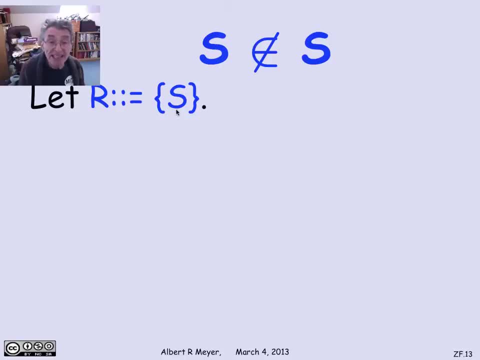 be a member of itself. Well, let r be the set consisting of just this set s that you're interested in. r is the singleton s. It's only element in s. Well, r is not empty And by the foundation axiom it must have. 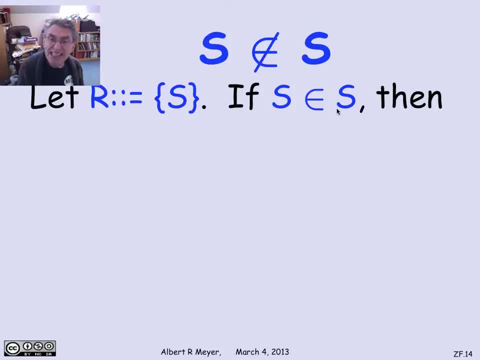 a membership minimal element. Now Suppose that s is in s. We're going to reach a contradiction. The claim is that r has no membership minimal element And that violates the foundation axiom. So you can't have s as a member of s. 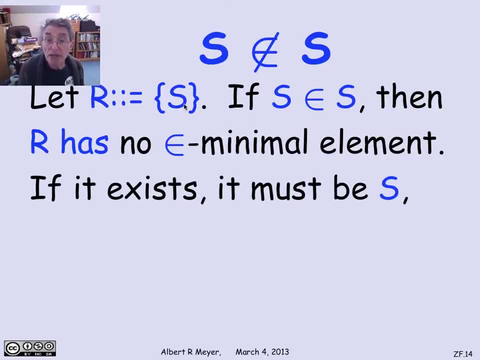 Why does this follow? Well, look, r is supposed to have a membership minimal element. Well, r's only got one element, So if it's got any membership element, it's got to be s. But s can't be membership minimal because s is in r. 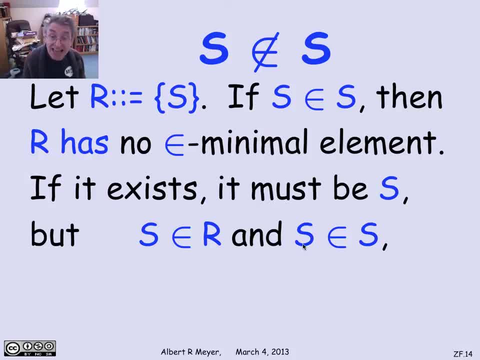 And it's got And And, which means that s has an element in r in it. So s is not r minimal, And the foundation axiom then immediately implies that you can't have s be a member of s. s is not membership minimal in r. 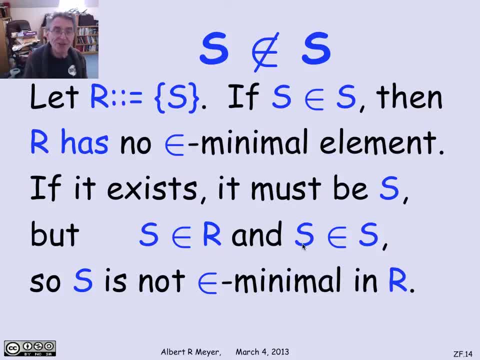 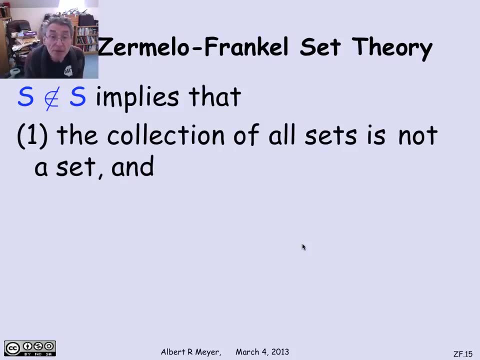 And this argument extends in a nice way to member of a member and member of a member, And we'll throw a feedback online question about that at you shortly. So, looking at the foundation axiom and the conclusion that no set is a member of itself, 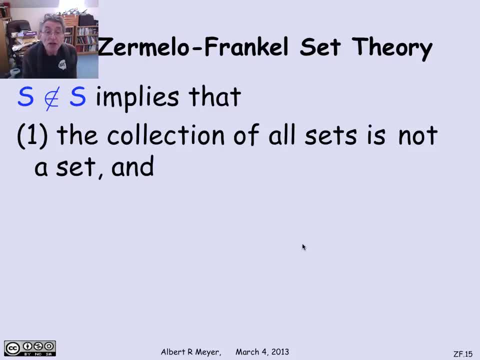 what we can immediately conclude is that, first of all, the collection of all sets can't be a set, Because if the collection of all sets was a set, then it would be a member of itself, And that's forbidden by the? s can't.